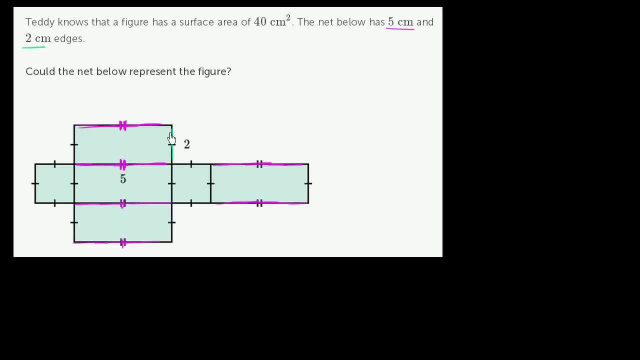 And then we have several 2 centimeter edges. So this one is 2 centimeters And any other edge that has the same number of hash marks- in this case 1, is also going to be 2 centimeters. So all of these other edges pretty much. 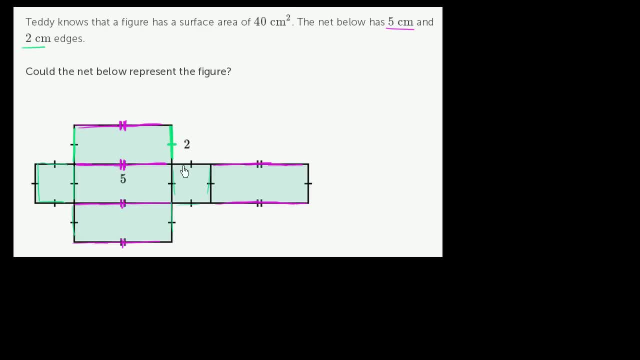 all the rest of the edges are going to be 2 centimeters. Now, they don't ask us to do this in the problem, But it's always fun to start with a net like this and try to visualize the polyhedron that it actually represents. 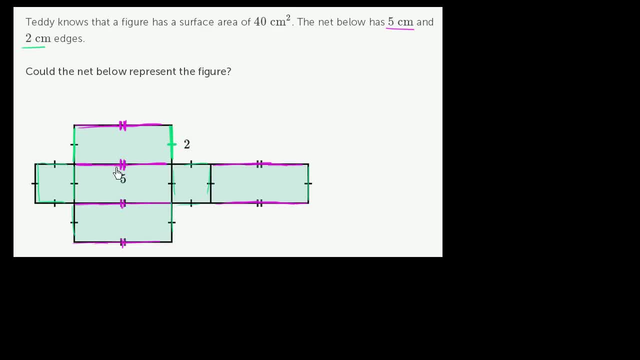 And it looks pretty clear. this is going to be a rectangular prism, But let's actually draw it. So if we were to- we're going to fold this in, We're going to fold this. that way, You could view this as our base right over here. 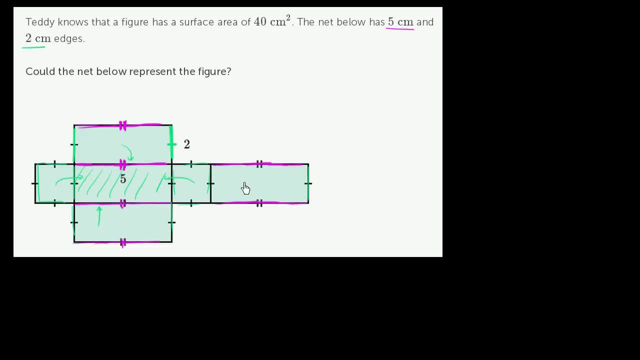 We're going to fold this in, We're going to fold that up, And then this is going to be our top. This is the top right over here. This polyhedron is going to look like this. This is going to look like this: 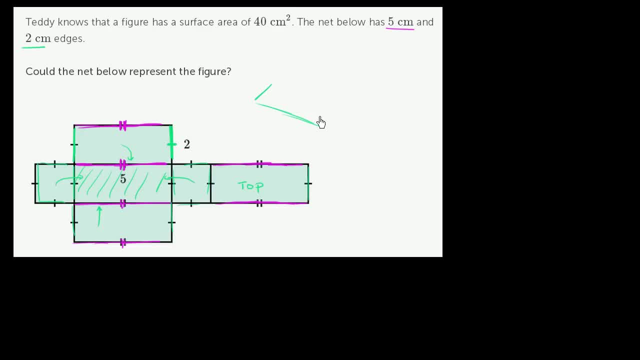 This is going to look like this. This is going to look something like this. So you're going to have your base that has a length of 5 centimeters. So this is our base. Let me do that in a new color. So this is our base right over here. 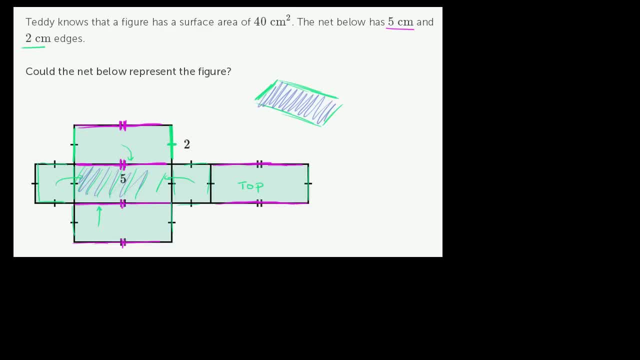 I'll do it in the same color. So that's our base, This dimension. right over here. I could put the double hash marks if I want, 5 centimeters, And that's of course the same as that dimension up there. 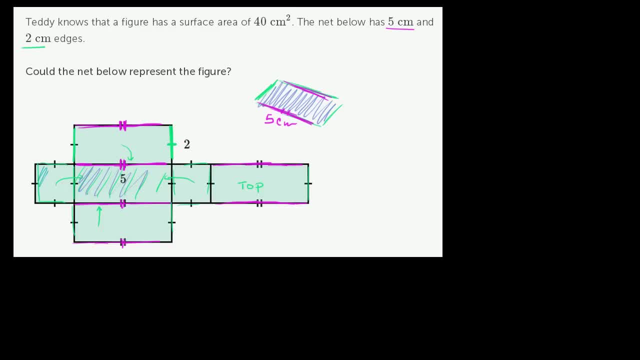 Now, when we fold up, When we fold up this side- let me do this in orange- actually, When we fold up that side, that could be this side right over here, This side right over here, along this 2 centimeter edge. 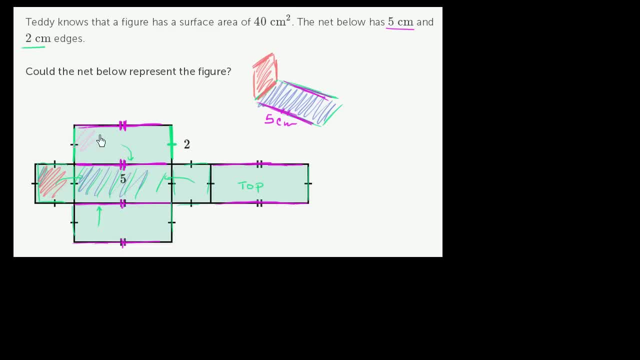 So that's that side right over here. When you fold this side in right over here, that could be that That's that side right over there, And then, when, of course, we fold this side in, that's the same color. 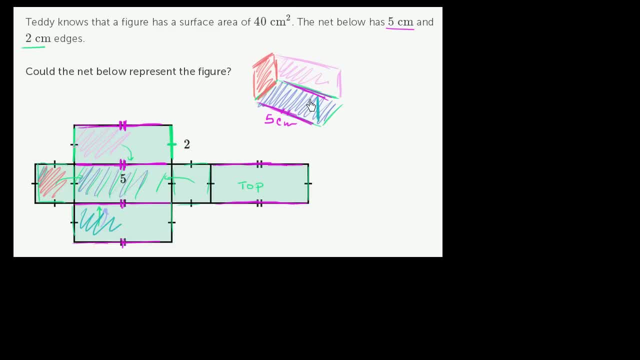 Let me do a different color. When we fold this side in, that's the side that's kind of facing us a little bit. So that's that right over there. That's that right over there. Color that in a little bit better. 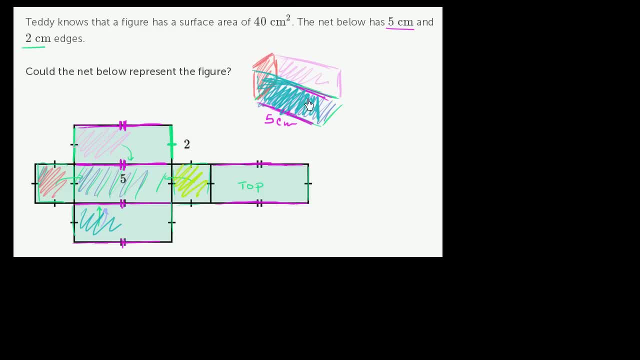 And then we can fold this side in, And that would be that side, And then, of course, we have the top. that's connected right over here, So the top would go. this would be the top, And then the top would, of course, go on top.